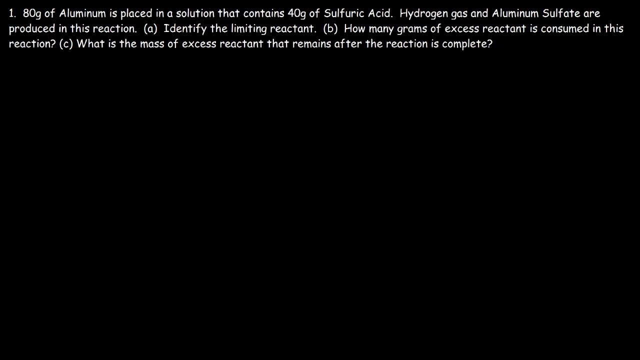 much is left over, So let's begin. The first thing we need to do is write a reaction and balance the equation. Aluminum is placed in a solution with sulfuric acid, Sulfuric acid is H2SO4 and it's going to produce hydrogen gas and 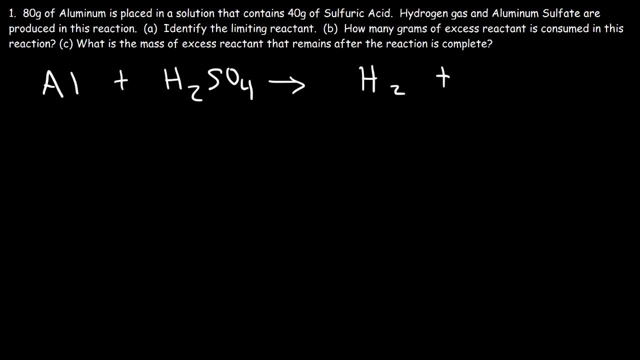 aluminum sulfate. Now what is the chemical formula of aluminum sulfate? Aluminum has a positive three charge, Sulfate has a minus two charge. So therefore the correct formula is Al2SO4 3.. Now we need to balance the chemical equation. 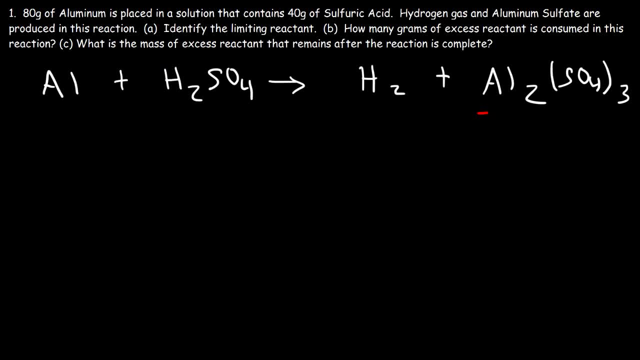 Notice that we have three sulfate ions on the right side and one SO4 unit on the left, So we got to put a three in front of H2SO4.. So we have three sulfate units Now we have two aluminum atoms on the right, so we need a two in front of Al. Now we have. 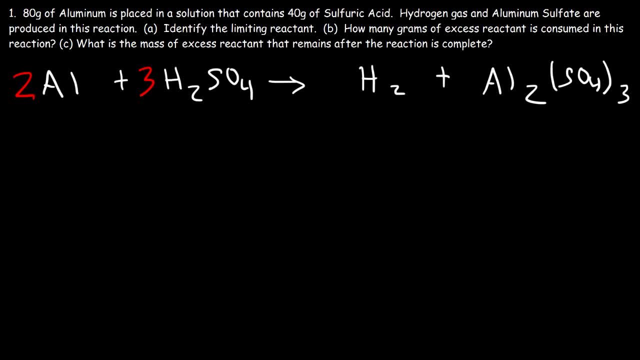 six hydrogen atoms on the left. so we got to put a three in front of H2 to have six hydrogen atoms on both sides. Now the equation is balanced. Let's put a one in front of this one. So 80 grams of aluminum is placed in a solution that contains 40. 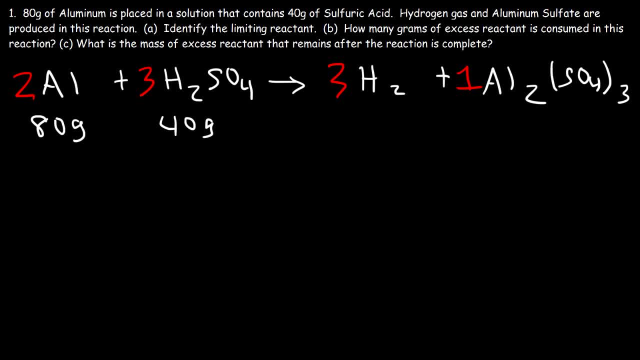 grams of sulfuric acid. If we're given the grams of each reactor, how can we find the limiting reactor? To do so, take the mass and divide it by the molar mass. The molar mass of aluminum is 26.98.. When you divide the mass by the molar mass, 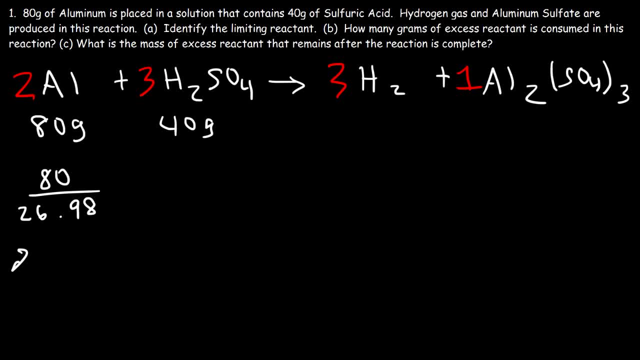 this will give you the number of moles. So we have 2.965 moles of aluminum. Now let's find the molar mass of H2SO4.. So there are two hydrogen atoms, one sulfur atom and four oxygen atoms. So 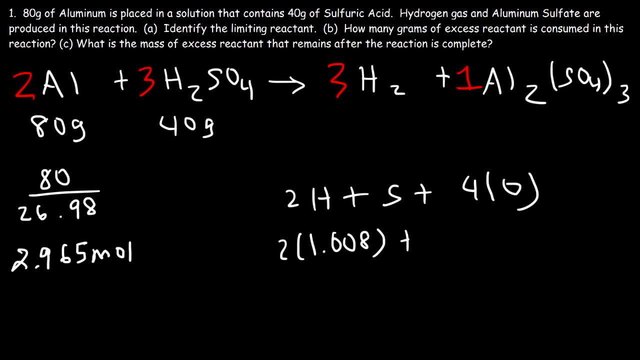 that's 2 times 1.008.. Sulfur is 32.07 and oxygen has an atomic mass of 16.. So four times 16, that's 64, plus 32.07, plus 2 times 1.008.. So the molar mass of H2SO4 is 98.086.. So let's 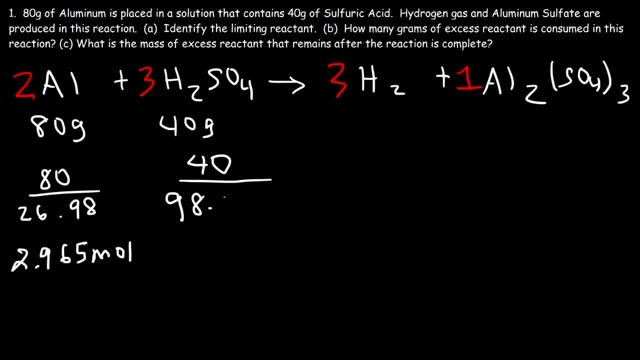 take 40 and divide it by that number, So this will give us 0.086.. So now what we need to do. clearly, we can see that the limiting reactor is going to be sulfuric acid. It's a lot less than aluminum, So what we need to do now is divide by the. 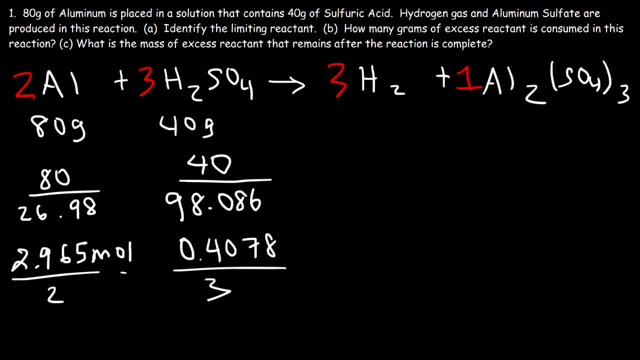 coefficient. If we divide 0.4 by 3, we're going to get a smaller number than aluminum. So Sulfuric acid has the lowest mole per coefficient ratio. So therefore H2SO4 in this example is the limiting reactant. 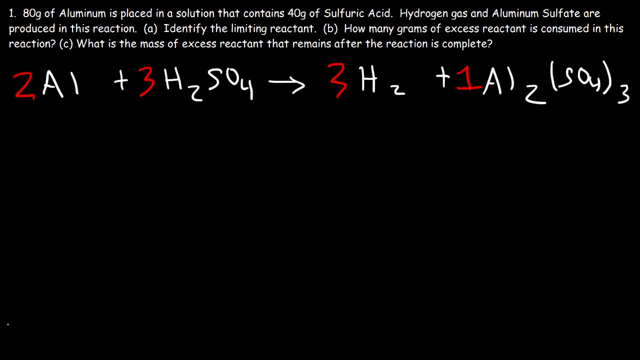 So now that we finished part A, let's move on to part B. So I'm going to write this as the limiting reactant, which means aluminum, is the excess reactant. Now, how many grams of the excess reactant is consumed in a reaction? 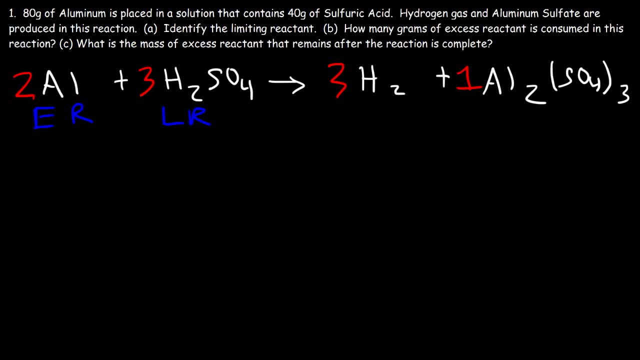 To do that you need to do a gram-to-gram conversion. Convert the grams of the limiting reactant to the grams of the excess reactant. This will tell you how many grams of the excess reactant is consumed in a reaction. So let's start with the 40 grams of sulfuric acid. 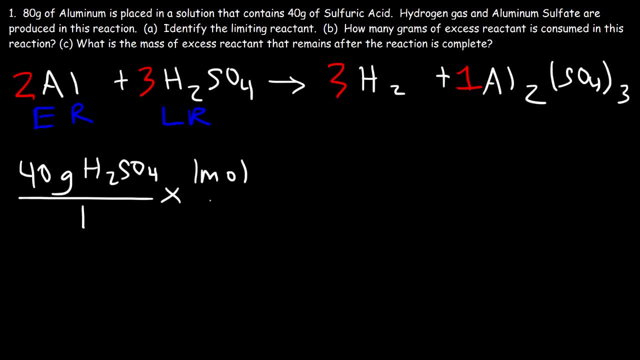 And let's convert it to moles. Now the molar mass of sulfuric acid: we said it was 98. 0.096.. Now we need to change the substance. So let's use the molar ratio between sulfuric acid and aluminum. 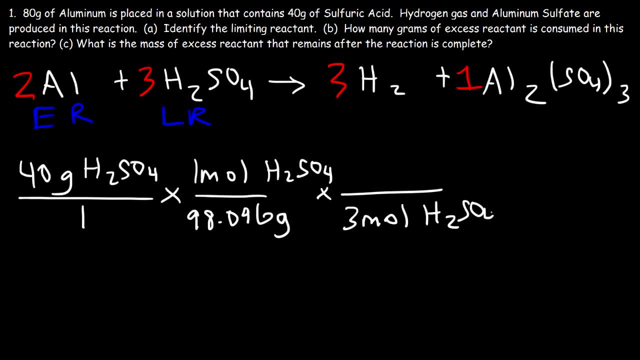 It's a 3 to 2 ratio. So for every 3 moles of sulfuric acid that reacts, 2 moles of aluminum reacts with it. Now let's convert Moles of aluminum to grams using the molar mass of Al, which is 26.98.. 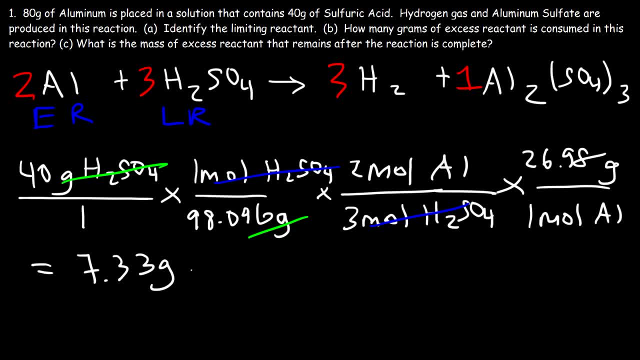 So I got 7.33 grams of aluminum. So this is the answer to part B, That is, the amount of excess reactant that is actually consumed in this reaction. So that's how much aluminum is used up in this reaction. So if 7.33 grams of aluminum is consumed in a reaction, 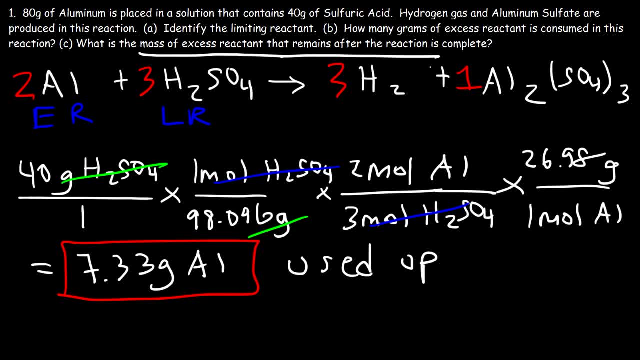 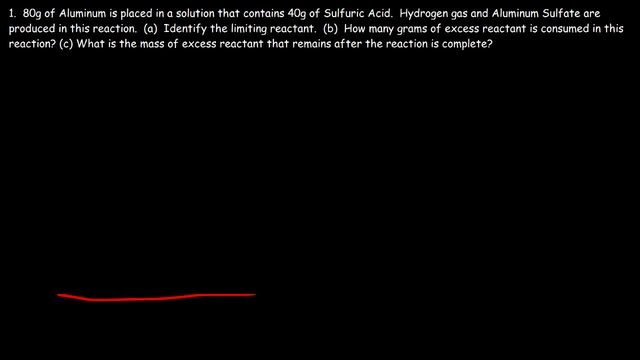 what is the mass of the excess reactant that remains after the reaction is complete? Let's make some space. So we started with 80 grams of reactant. During the course of the reaction, 7.33 grams of aluminum was consumed. 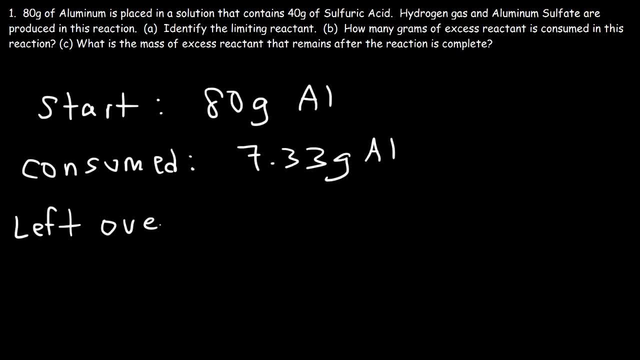 So the amount that's left over, or the amount that remains, is going to be the difference of 80 and 7.33.. So if we subtract those two numbers, this will give us the answer to part C. It's 72.67 grams of aluminum. 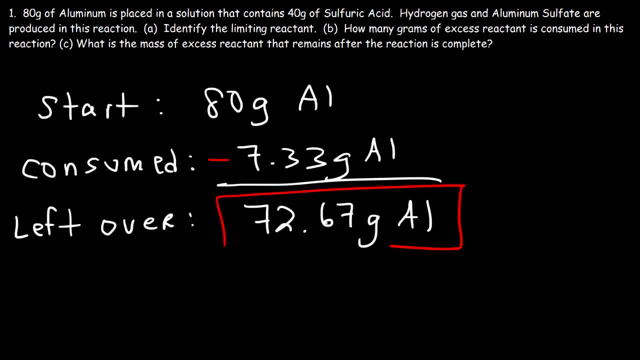 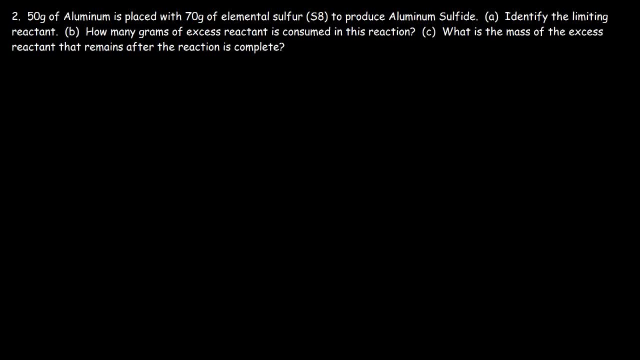 So that's how much excess reactant remains after the reaction. That's how much is left over For practice. go ahead and try this one. See if you understand this concept. Feel free to pause the video and see if you can get the right answer. 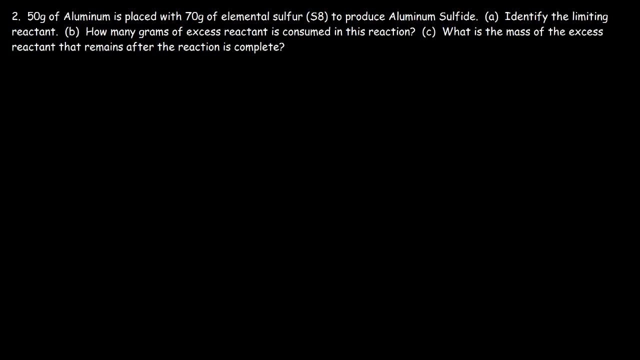 So 50 grams of aluminum is placed with 70 grams of elemental sulfur S8, to produce aluminum Sulfide. Identify the limiting reactant. So we have aluminum reactant with sulfur And it produces aluminum sulfide. Now what is the chemical formula of aluminum sulfide? 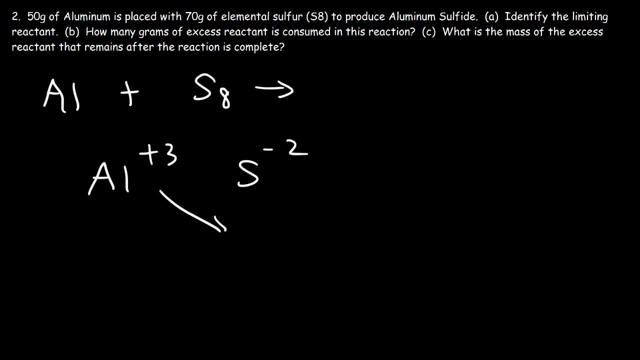 Aluminum has a positive 3 charge. Sulfur has a negative 2 charge, So it's going to be Al2S3.. Now we need to balance the chemical equation. The least common multiplier between 8 and 3, or just 8 times 3, is 24.. 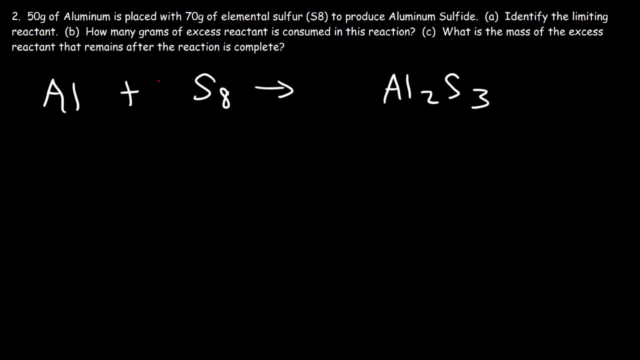 So we need 24 sulfur atoms on both sides. Let's put a 3 in front of S8 and an 8 in front of Al2S3.. So we have 24 atoms of sulfur on the left and on the right side. 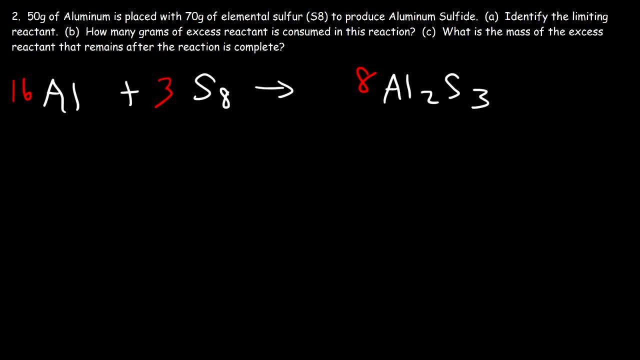 Now 8 times 2 is 16. So we need a 16 on the left. So now the number of aluminum and sulfur atoms are the same on both sides. Now we're mixing 50 grams of aluminum, 50 grams of aluminum, with 70 grams of sulfur. 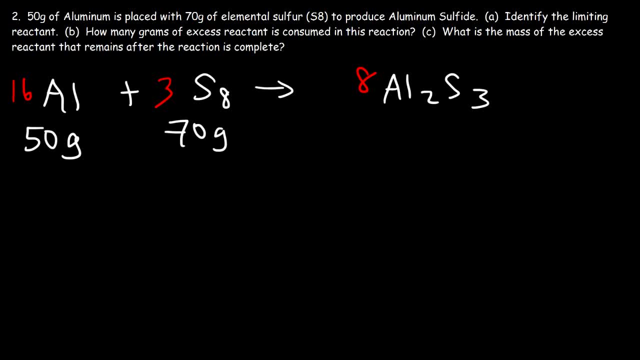 Which one is going to be the limiting reactant? Is it the one that has less grams or more grams? Is it aluminum or sulfur? What do you think? Well, first, let's find the moles of each substance. So let's take the grams and divide it by the molar mass. 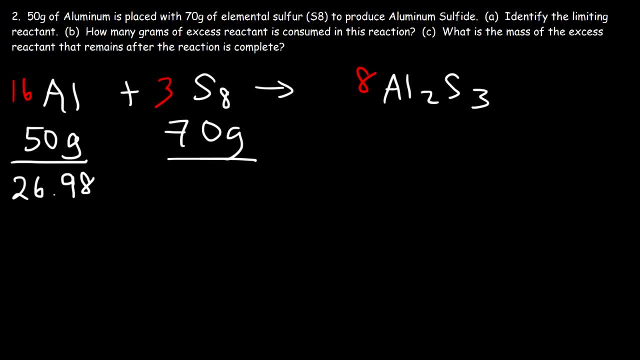 The molar mass of aluminum is 26.98.. And for sulfur it's going to be 8 times the atomic mass of sulfur, which is 32.07.. So the molar mass of the S8 molecule is 256.56.. 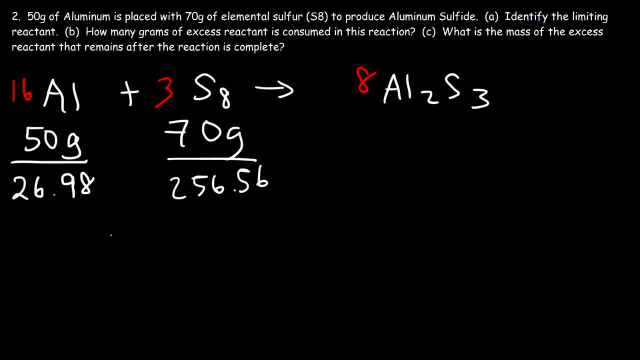 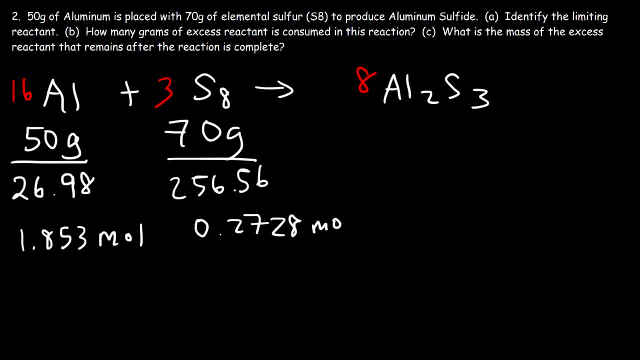 That's 0.2728 moles. So which one do you think is the limiting reactant at this point? Is it aluminum or sulfur? We have a lot more moles of aluminum, But let's see. Now that we have the quantity of aluminum and sulfur, we'll need to divide it by the. 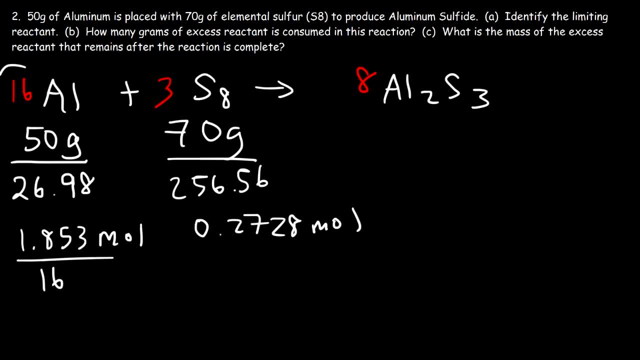 coefficient. The coefficient in front of aluminum is 16.. In front of sulfur it's 3.. So 0.2728 divided by 3 is 0.2728.. So 0.2728 divided by 3 is 0.2728.. 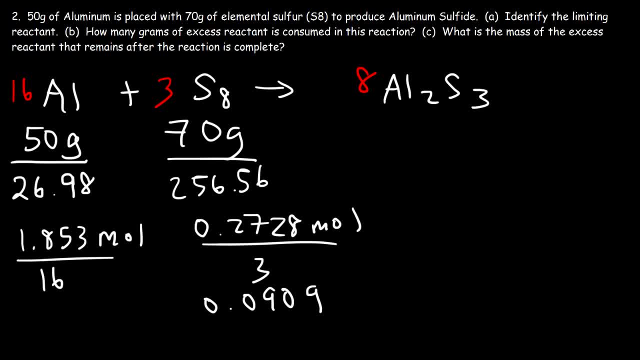 0.2728 divided by 3 is 0.2728.. 0.0909- 1.853 divided by 16, that's 0.1158. so in this case sulfur is the limiting reactant. it's close to aluminum but it has the lowest mole per. 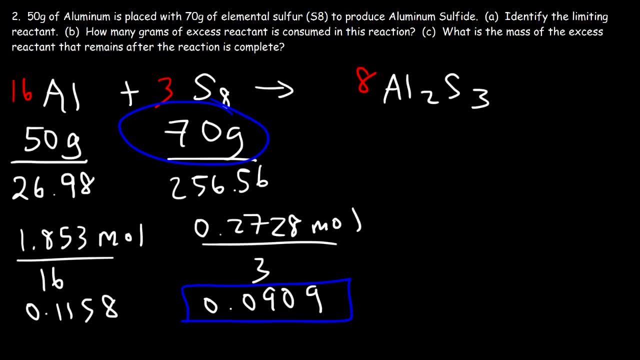 coefficient ratio. so even though we had a greater amount of mass of sulfur doesn't mean it was a limiting reactant. you can't look at the grams and determine the limiting reactant. you need to find the lowest mole per coefficient ratio. now let's move on to the next part: how many grams of excess reactant is? 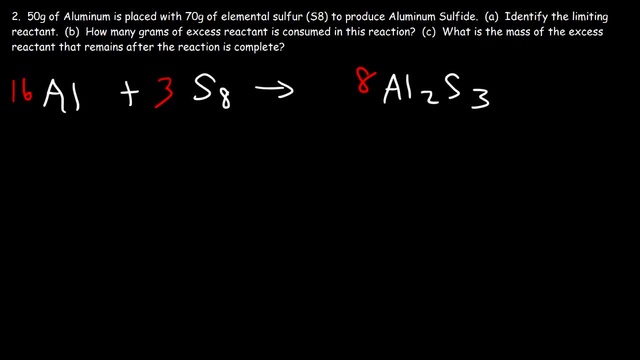 consumed in this reaction. so we know this is the limiting reactant and this is the excess reactant. to answer part B, take the grams of the limiting reactant and convert it to the grams of the excess reactant. if you do it this way, the grams. 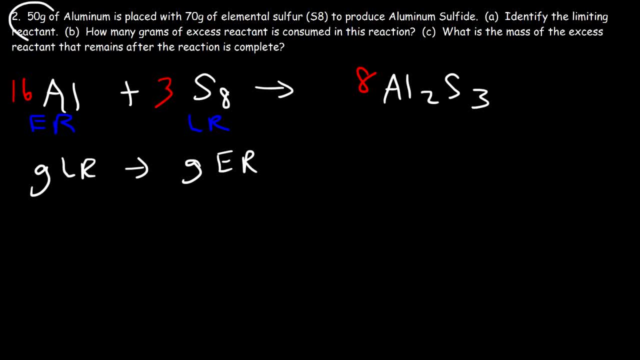 of excess reactant that you get should be less than how much you started with. if you try to do it the other way, you probably get more than the other reactant. so just always start with the limiting reactant. so we're going to start with 70 grams of elemental sulfur and let's convert it to moles. so we know. 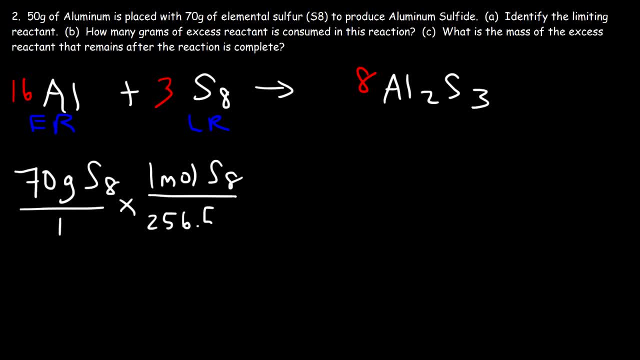 that the molar mass is 256.56. and now let's change the substance from the limiting reactant to the excess reactant using the molar ratio. so for every three moles of sulfur that reacts, 16 moles of aluminum will react with it. now let's 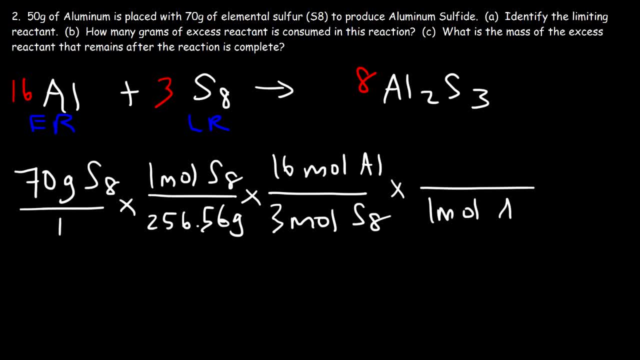 convert moles of aluminum to grams using the atomic mass of aluminum, which is 26.98. so it's going to be 70 divided by 256.56, and then multiply that by 16 and divided by 3, and then multiply that result by 26.98, so this will give you 39.26 grams. 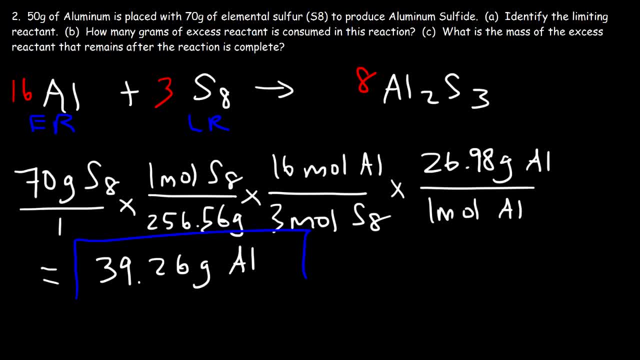 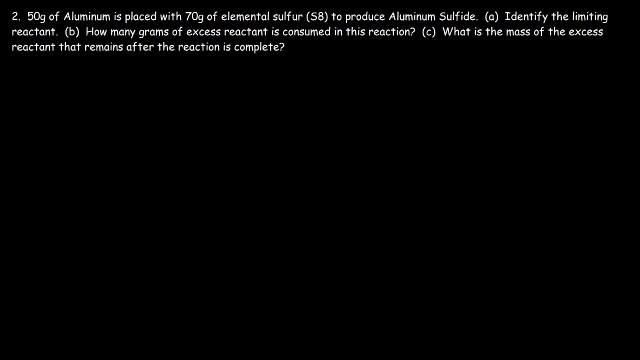 of aluminum. so this is the amount of aluminum that is consumed in a reaction. that's the answer for Part B. now let's move on to the last part. what is the mass of the excess reactant that remains after the reaction is complete? so the excess reactant is aluminum. we started with 50.